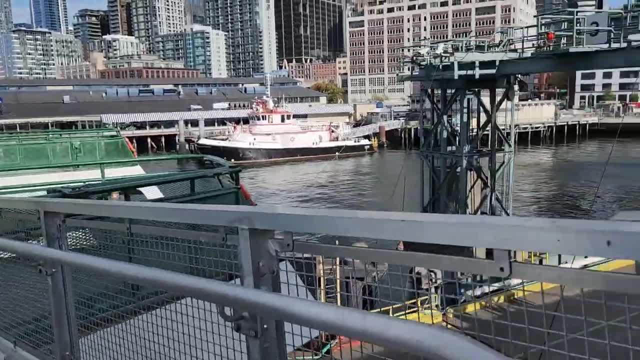 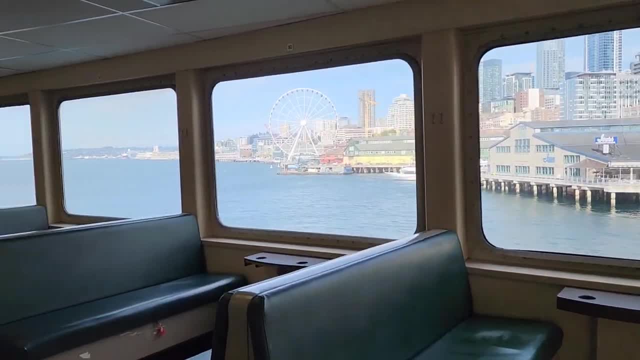 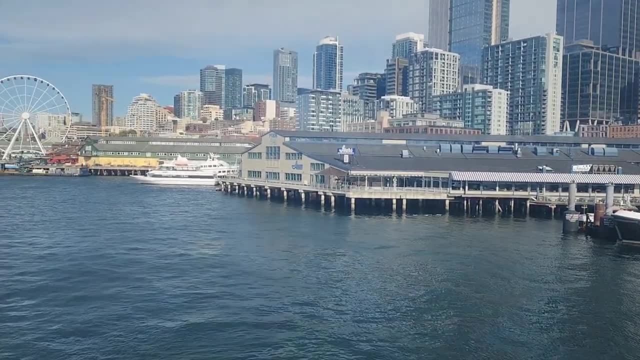 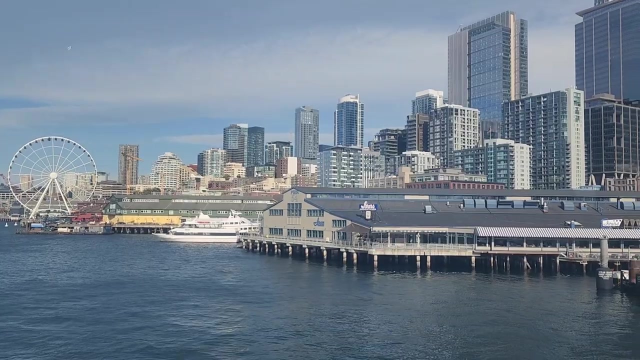 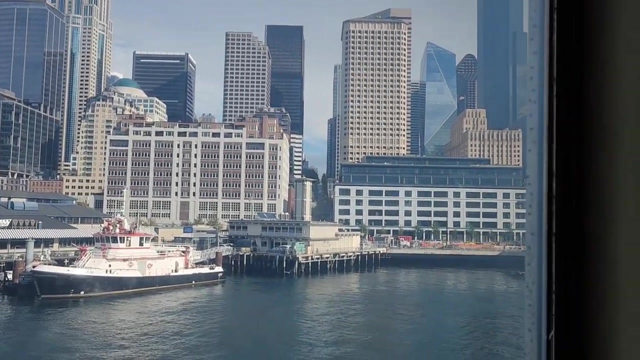 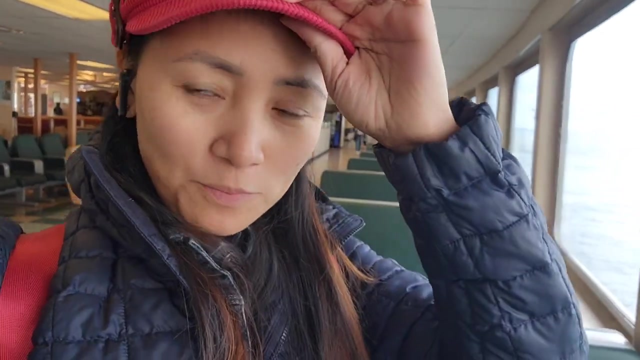 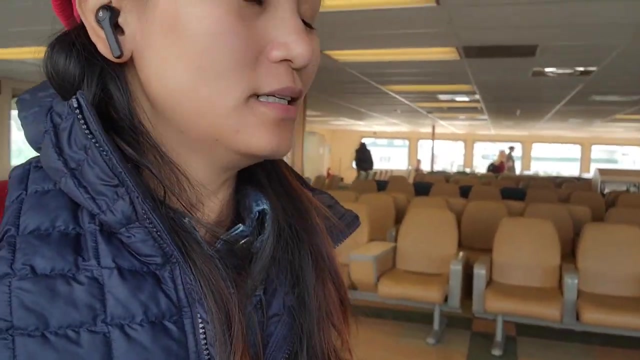 3. 1., 2. 3.. Oh my gosh, this is so cool. Wow, look at this. It's amazing. This is Seattle, Seattle, And this is me heading back to Port Orchard, And it's a big ferry. Let's go. 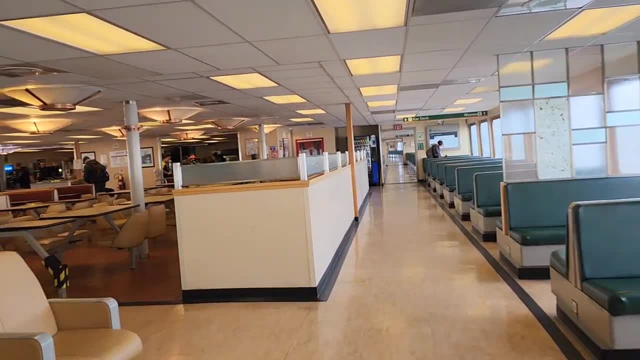 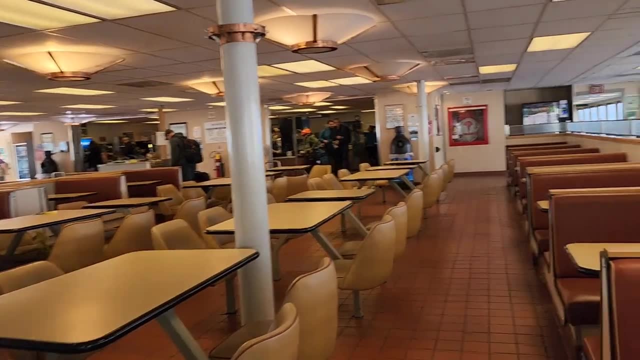 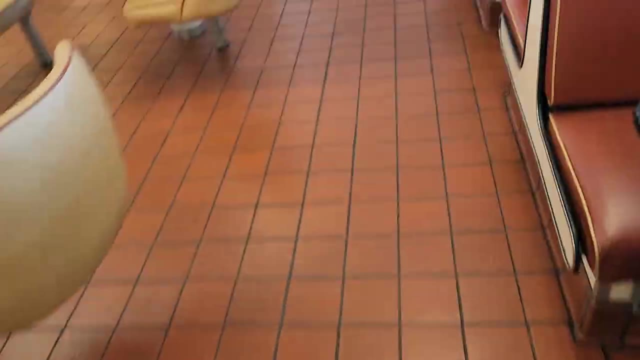 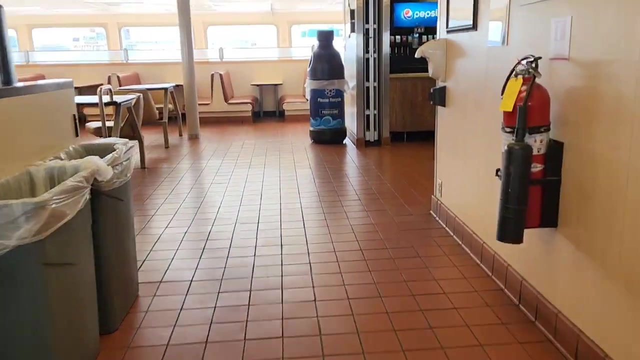 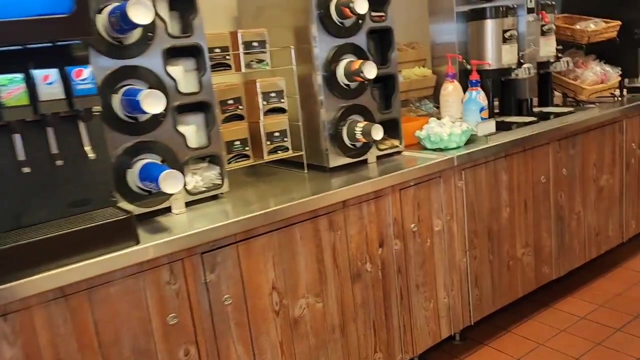 walk around Let's see what they have here. I think they have some food. Probably can order some. Let's see what they have for food. My noisy suitcase- Wow, They have. oh, Really cool, They have some good stuff. 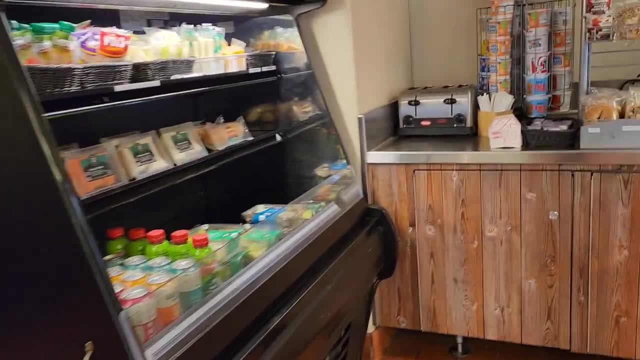 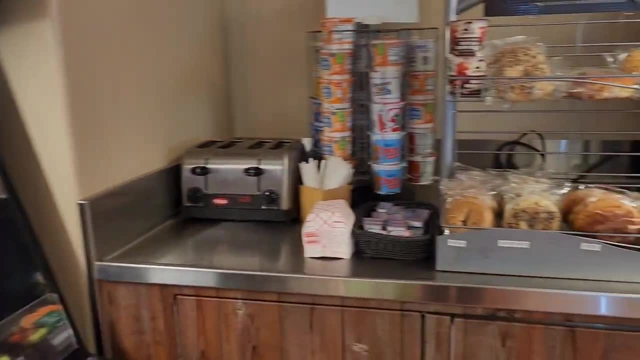 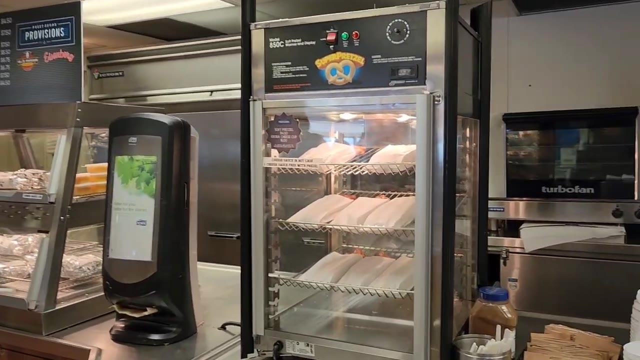 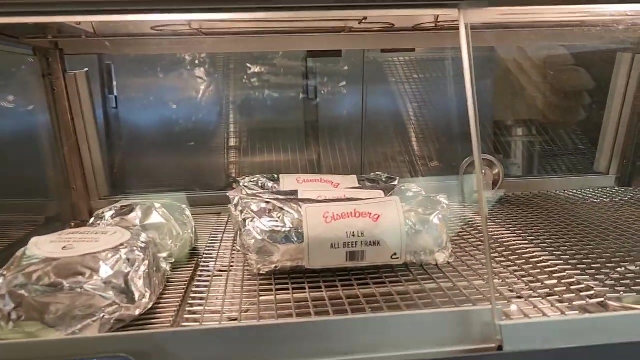 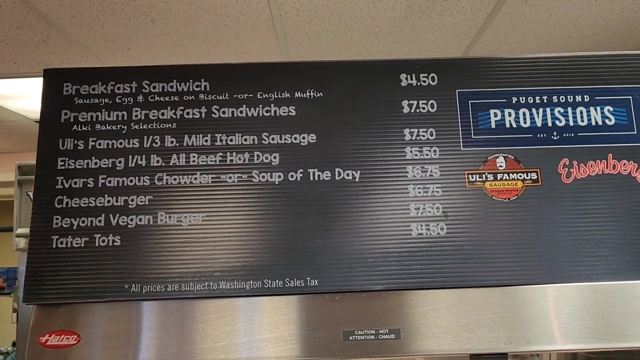 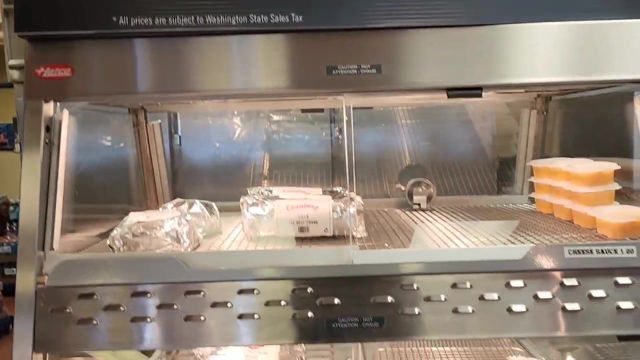 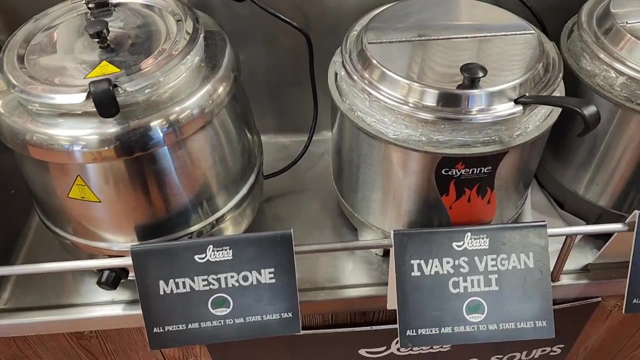 Popcorn- What else? Salad Or bagels? How do they get food soon? Wow, Might get some plant-based bacon. Wow, that's their price. Wow, Sandwich Cheeseburger- I might just get a cheeseburger, Some kind of hat. 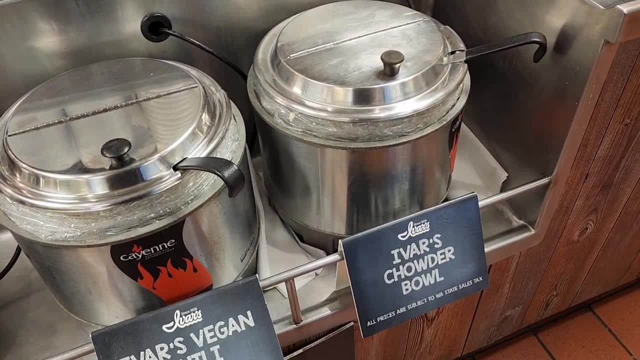 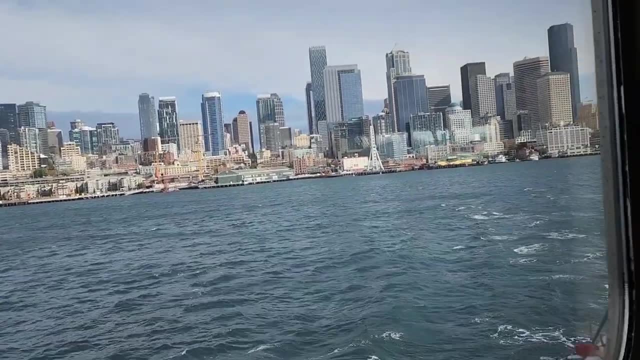 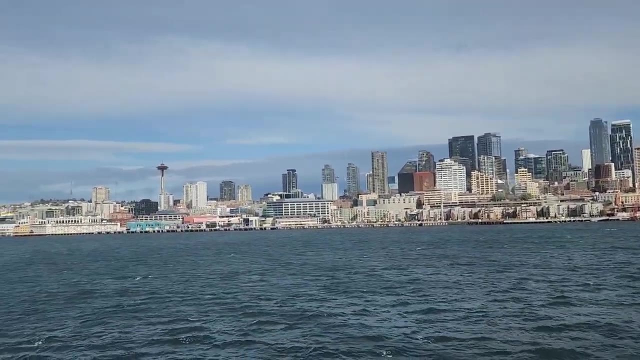 I think I'm going to get some of that Ivar's charger bowl, So leaving Seattle. Look at that, It's so gorgeous. It's a gorgeous day. It's chilly, Windy. I'm going to go check the outside. 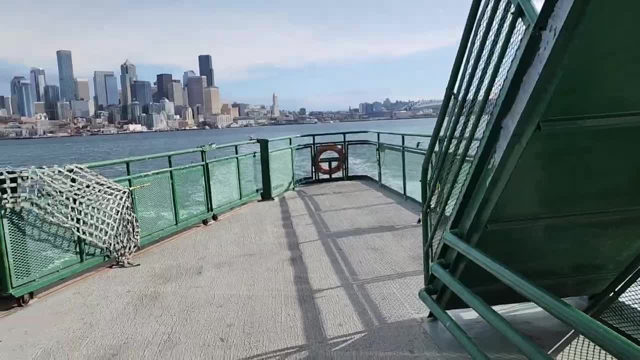 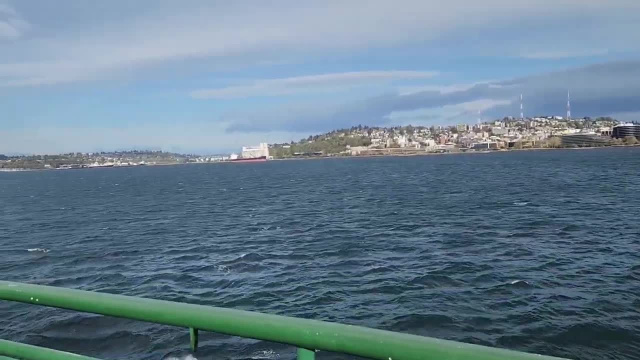 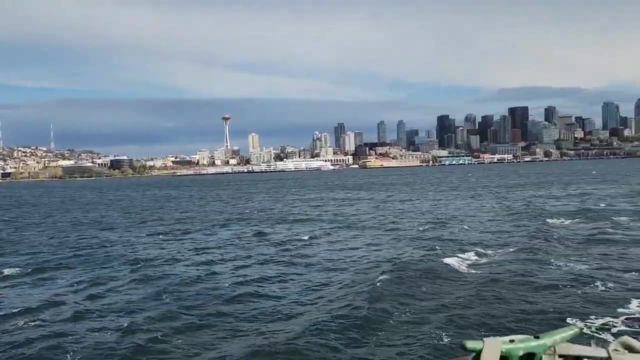 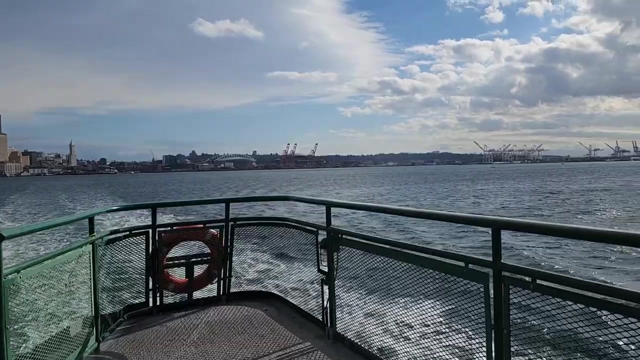 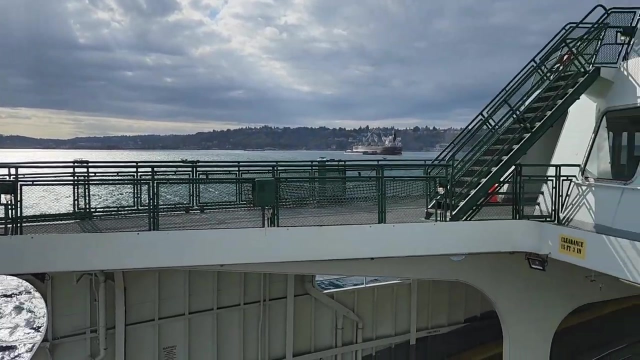 Whoa, There it is. I'm on a ferry to Bremerton And this is not a fast ferry. It's like an hour to get there. But wow, Look at this, It's so cool. Okay, Not many cars in there. 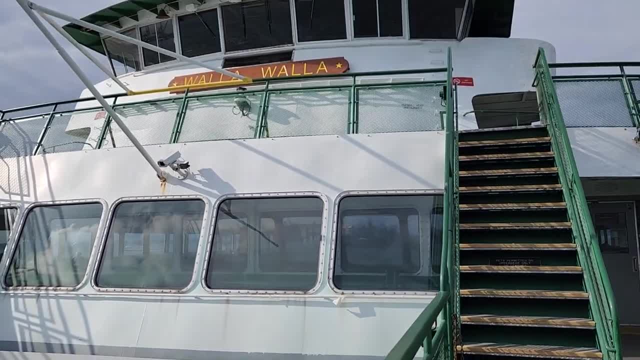 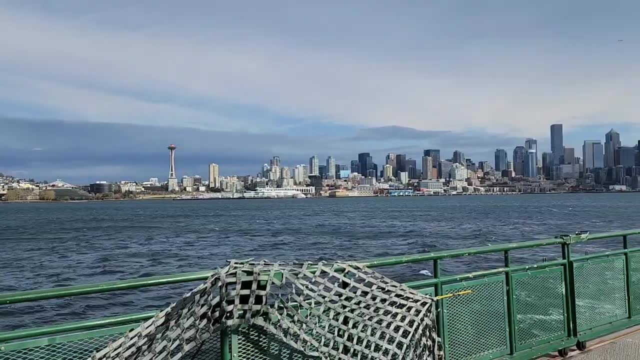 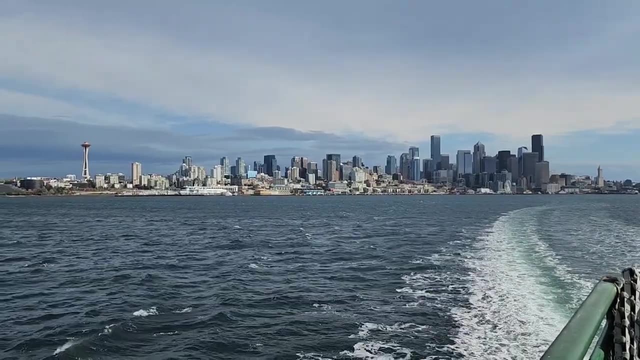 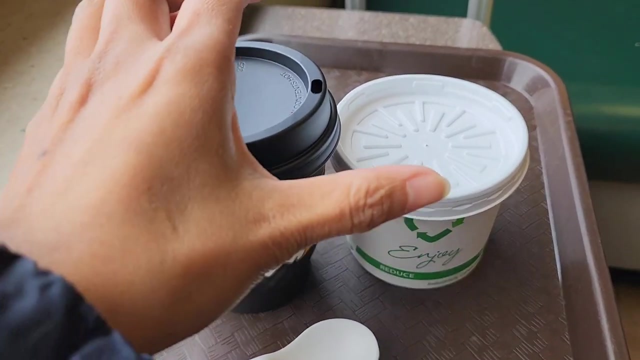 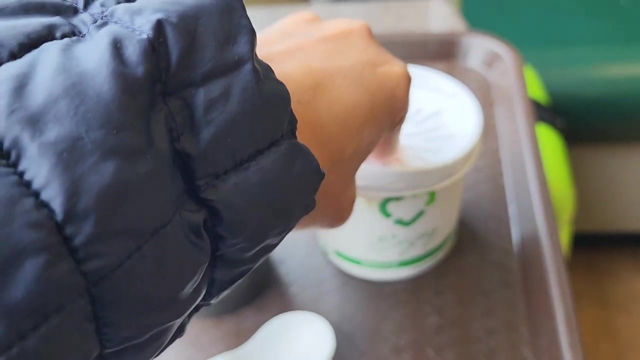 You don't even see any Walla, Walla, Walla, Walla. There it is. Yeah, Bye Seattle, Until next time. Here's what I got: Coffee and a clam chowder- Ivar's clam chowder. 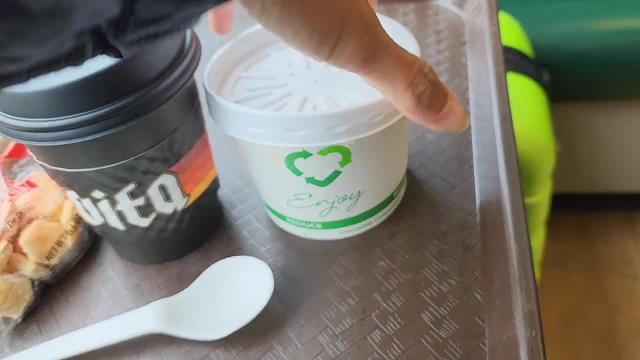 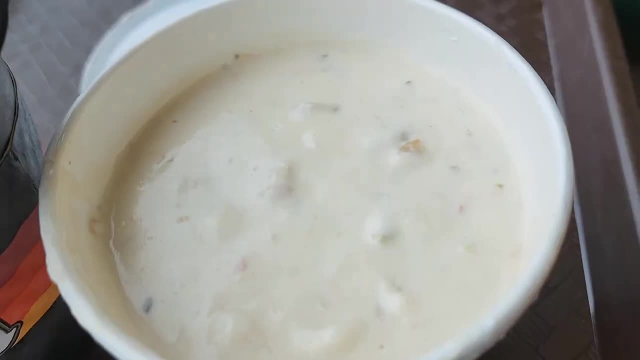 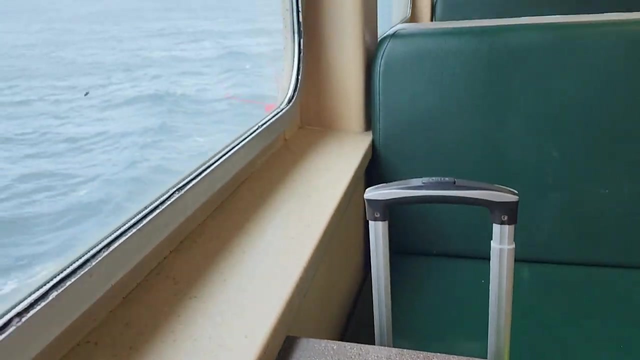 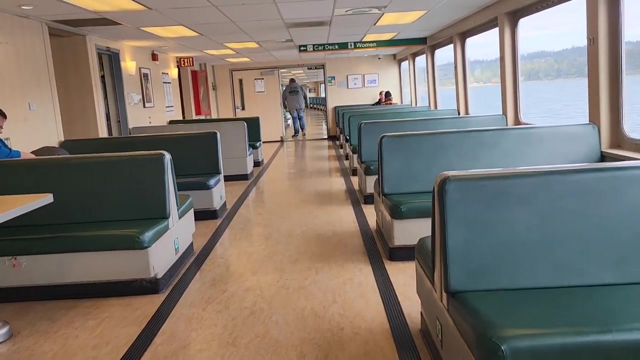 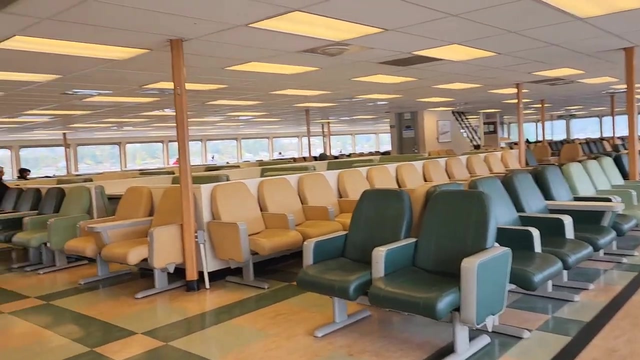 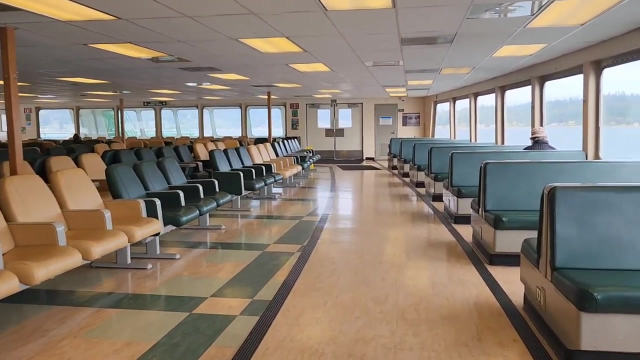 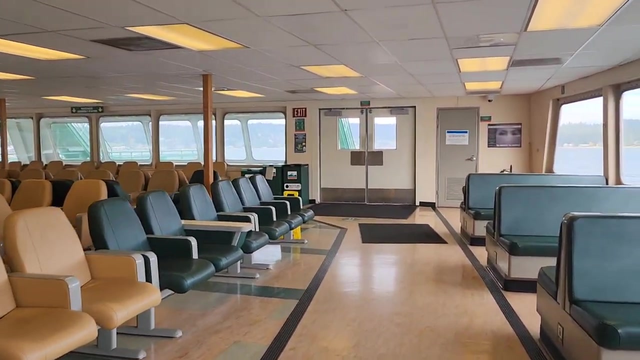 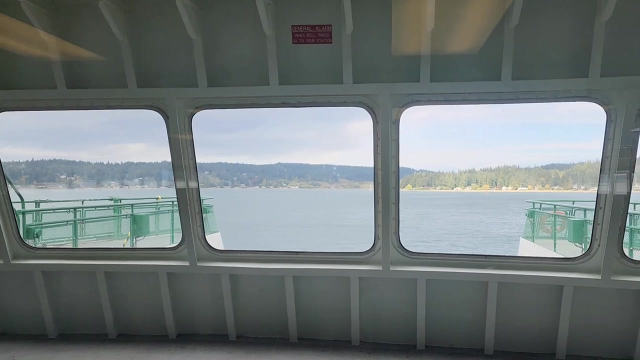 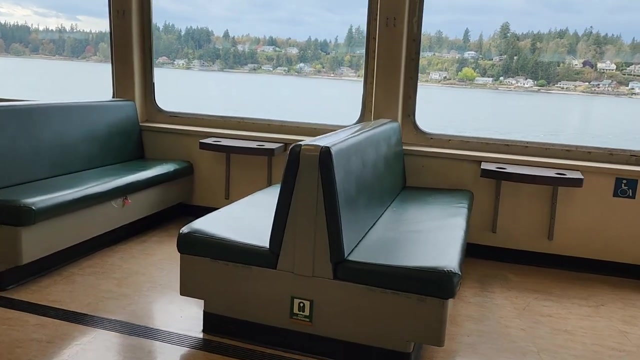 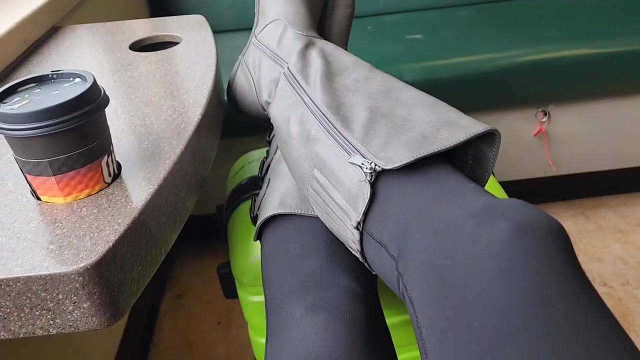 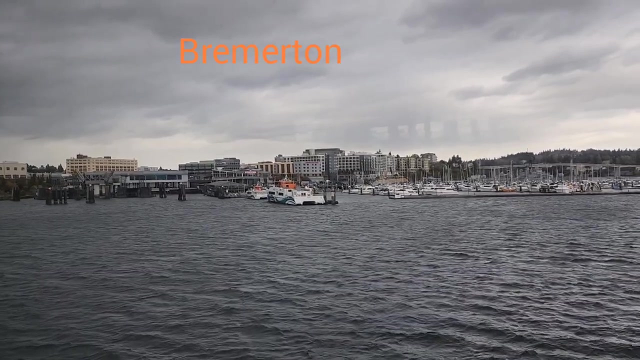 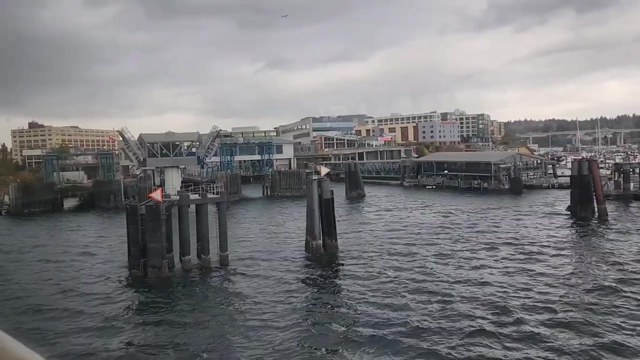 It's a famous clam chowder. Yes, Nice Warm In this cold weather. That's so many people, Not so many passengers here. Let's see here what. Let's see here what. Your attention, please. Destination, Please make sure. 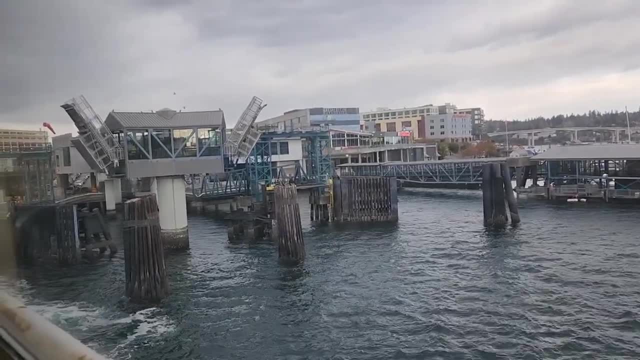 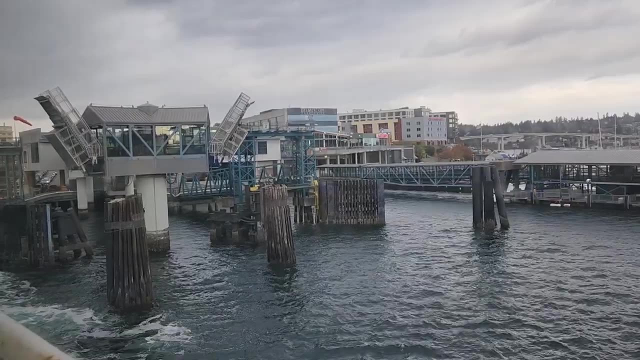 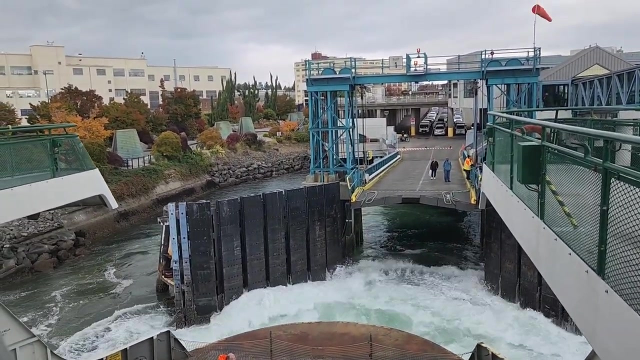 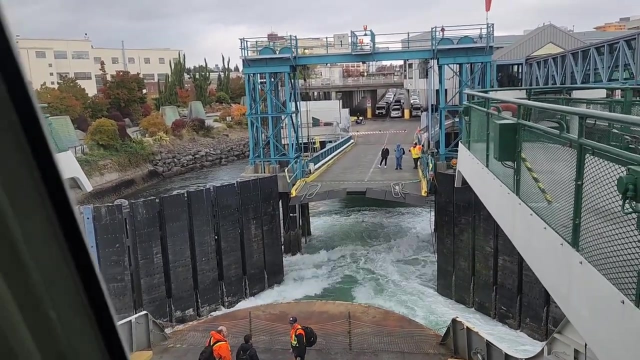 that you have all of your personal belongings before you disembark on the vessel. Drivers and passengers return to your vehicle. For safety and health reasons, do not start your engine until directed by a crew member. 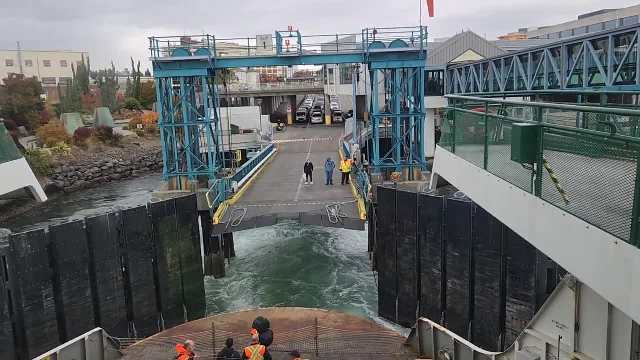 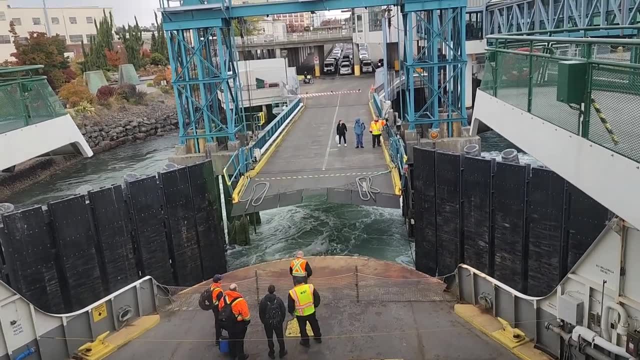 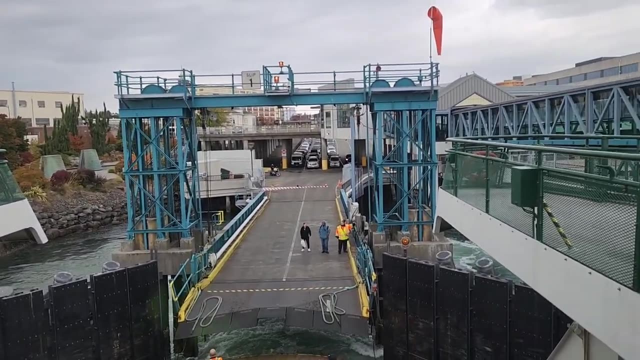 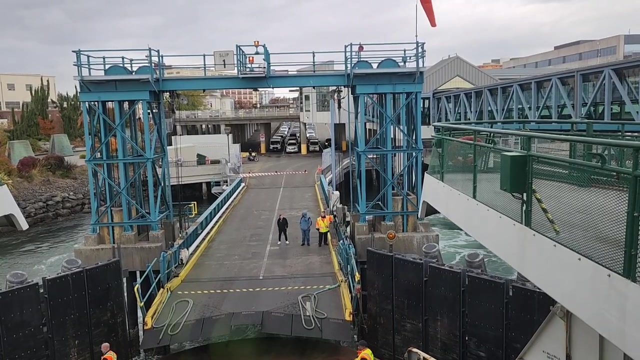 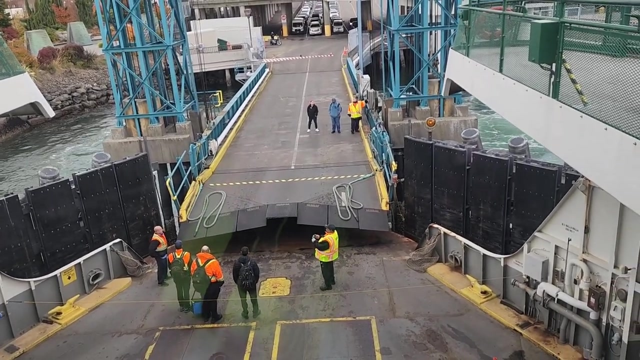 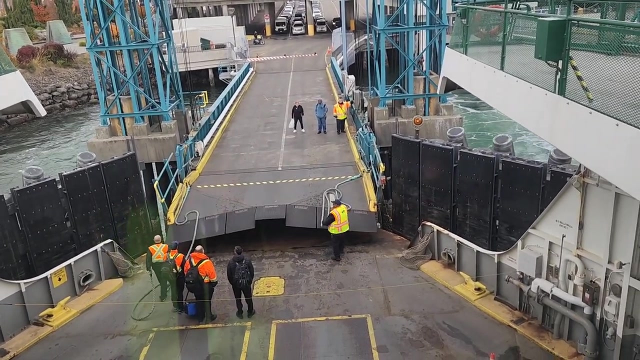 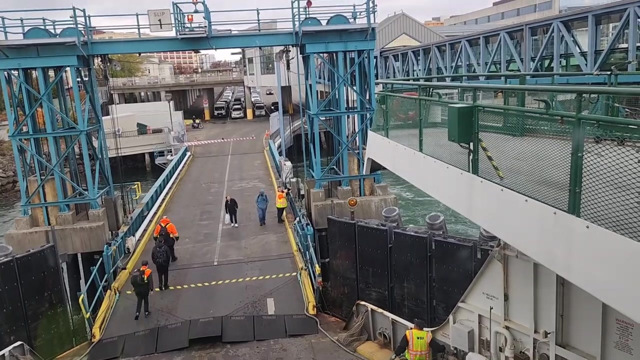 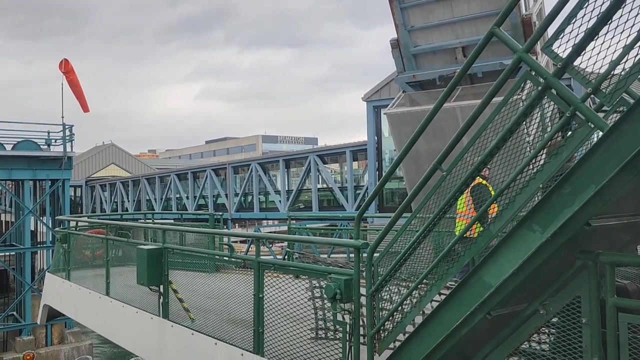 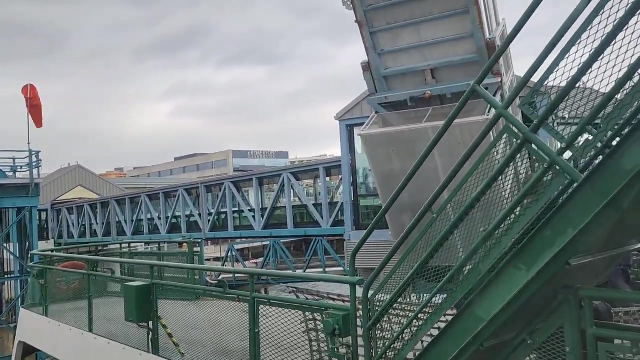 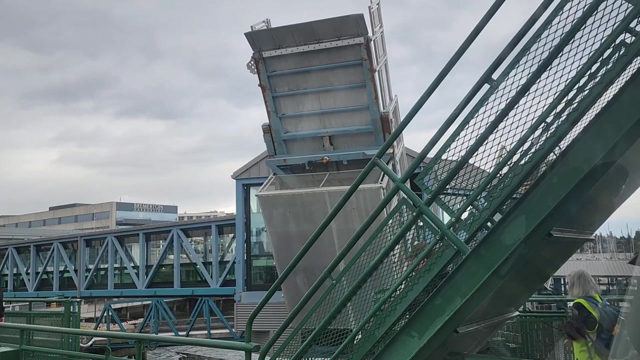 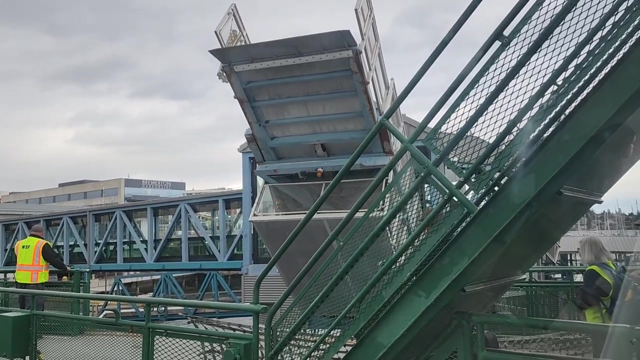 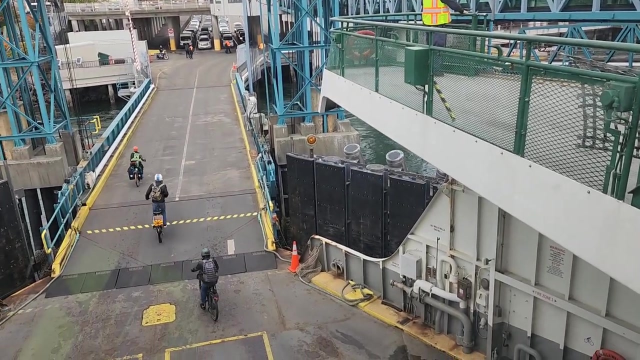 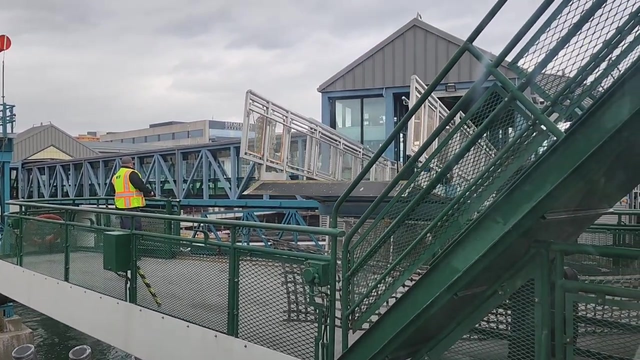 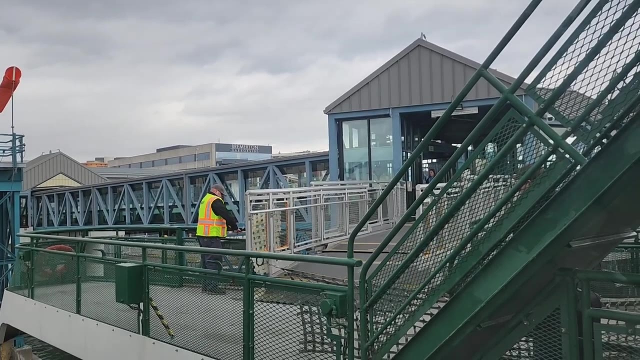 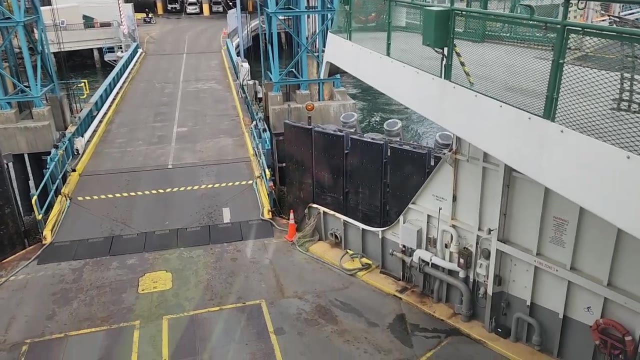 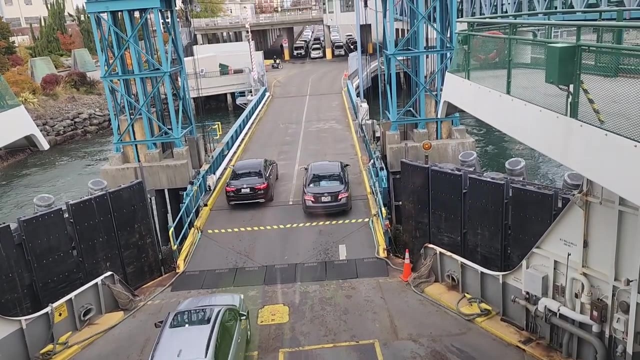 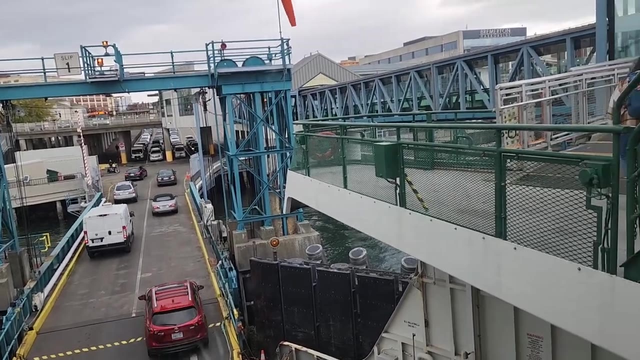 We are here. That is so cool. It only cost us $9.45 with a car and it's time for me to go because I have to catch on another. 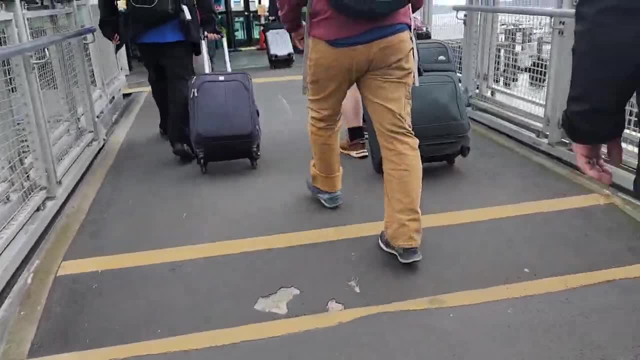 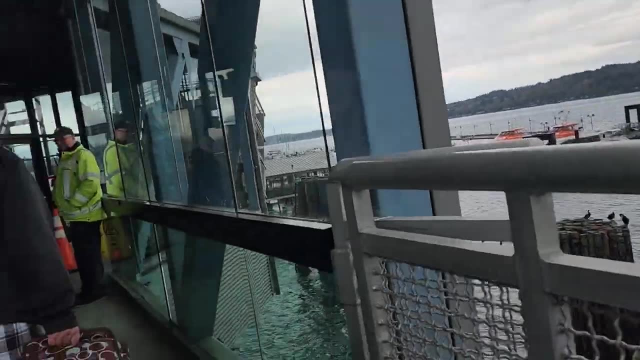 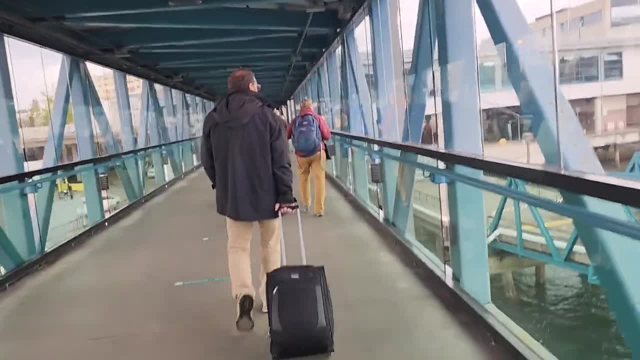 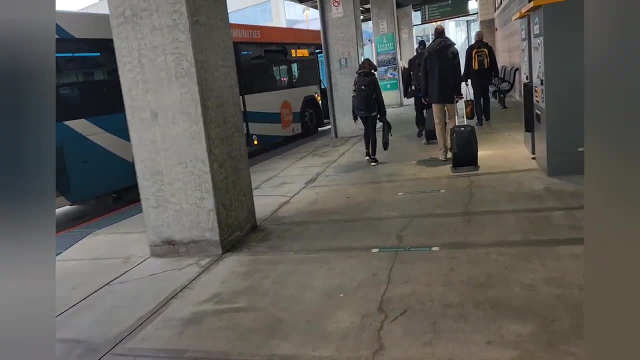 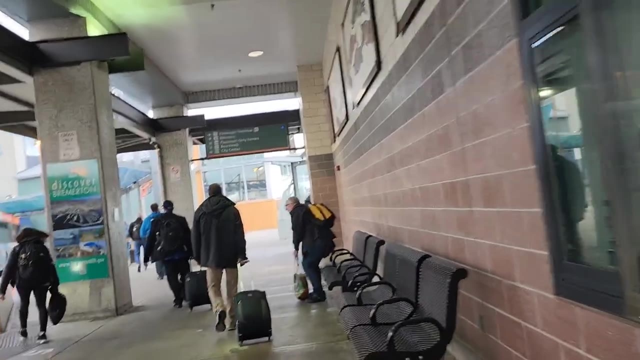 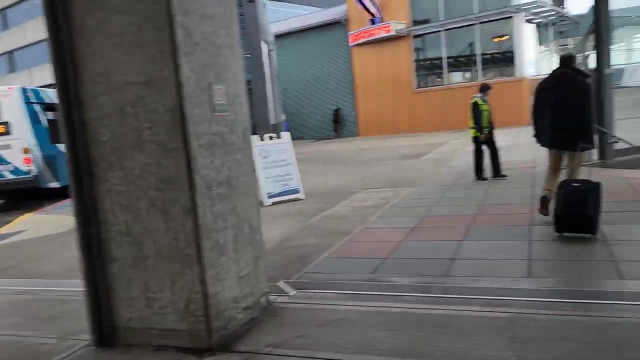 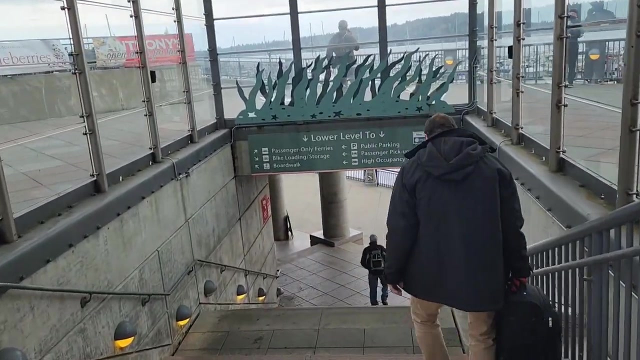 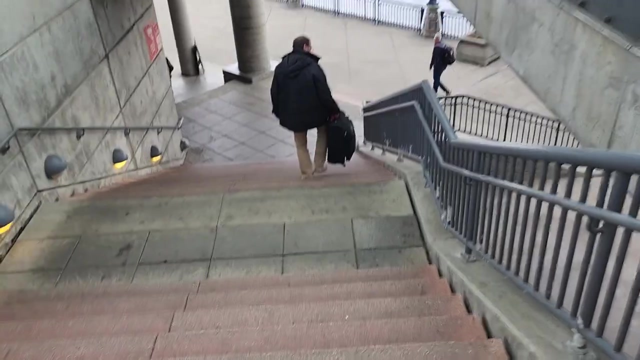 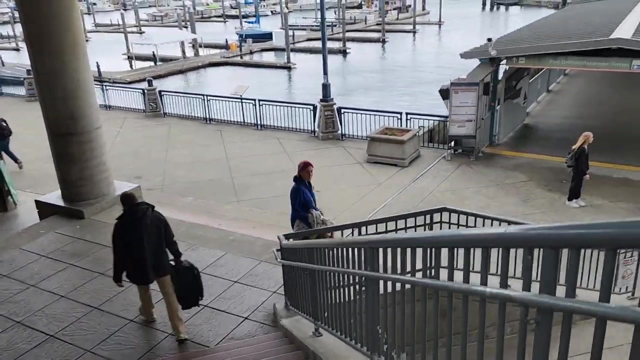 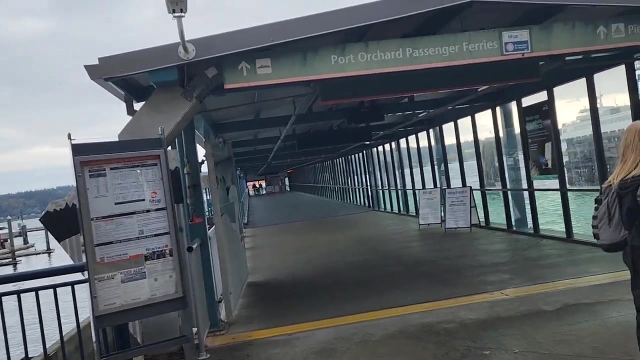 I just need to wait a couple minutes. right Buses. I have to get down to passenger terminal. What's this? It's red There we go another stairs. Good thing my suitcase is not too heavy. Oh, this is where we like to portal chart. Oh, $2.. So there's the ferry I was in. It cost $9.45 for an hour ride from Seattle to Birmingham. Now I'm going to portal chart and it cost me $2.. That's only like 15 minutes or less. 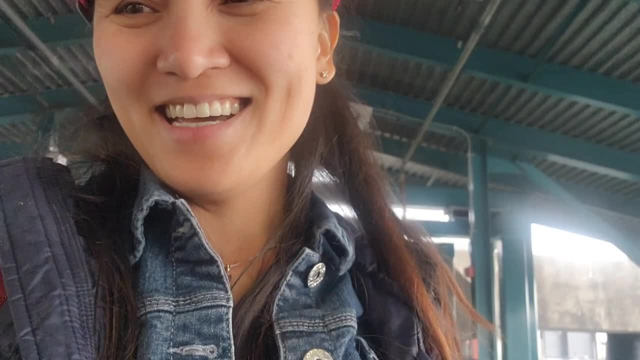 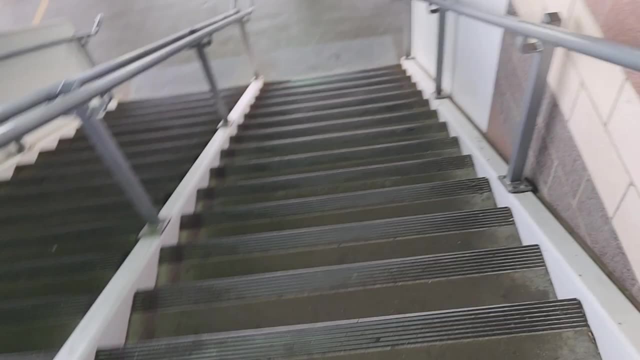 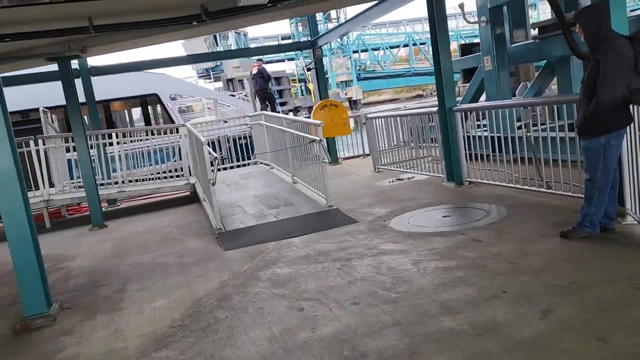 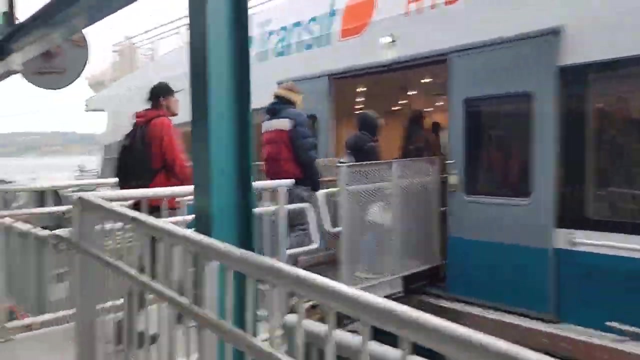 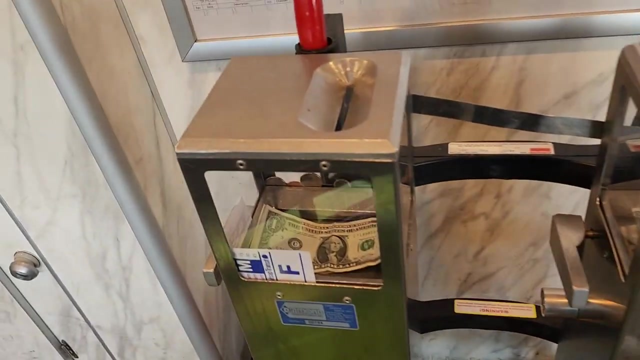 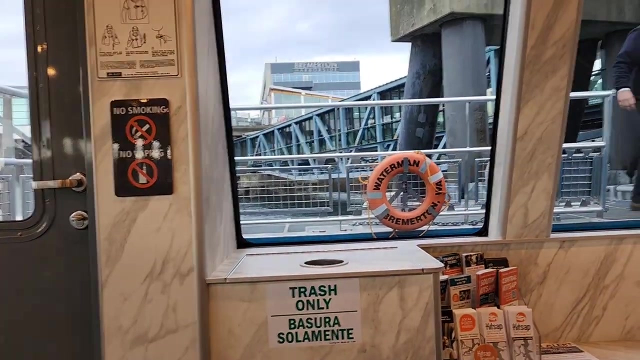 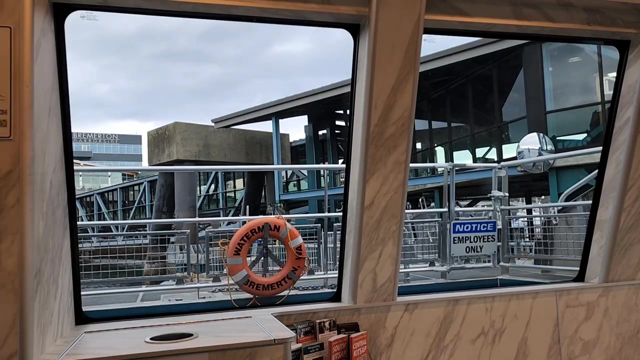 Guess what? It's? another stairs, Another stairs. It's not too heavy. There's the ferry from portal chart. So I'm going to portal chart. I'm going to portal chart. No, leaving for portal chart. It's almost 2 o'clock. 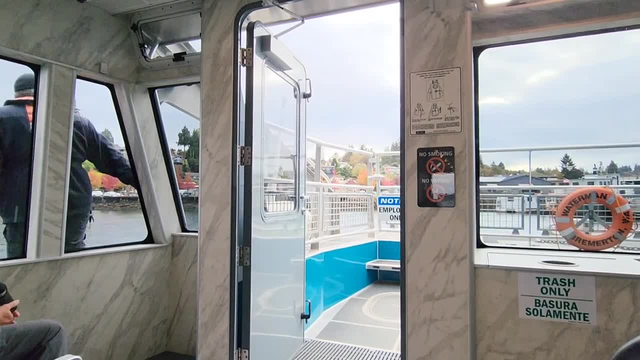 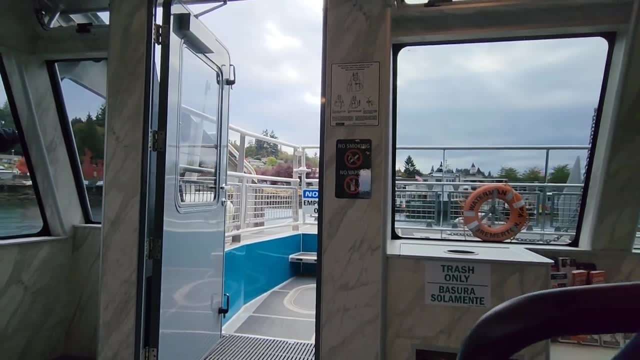 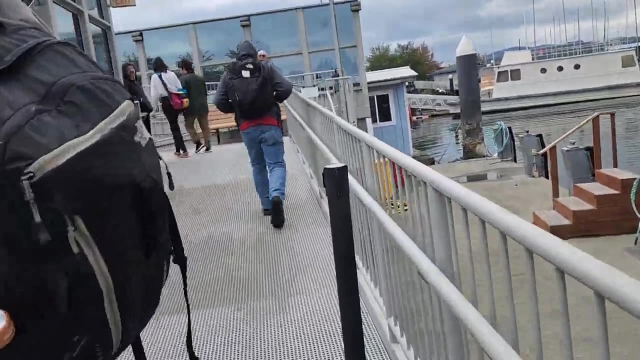 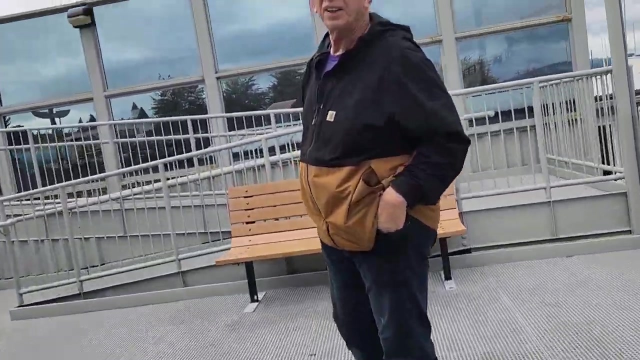 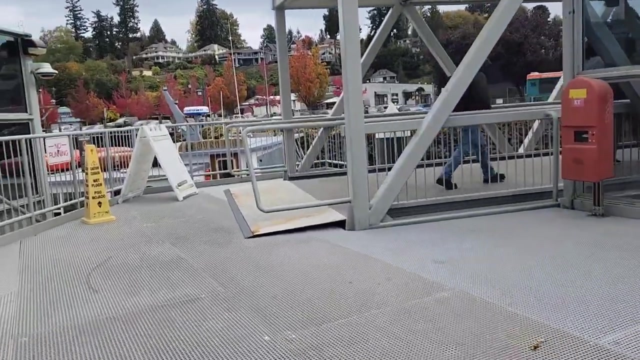 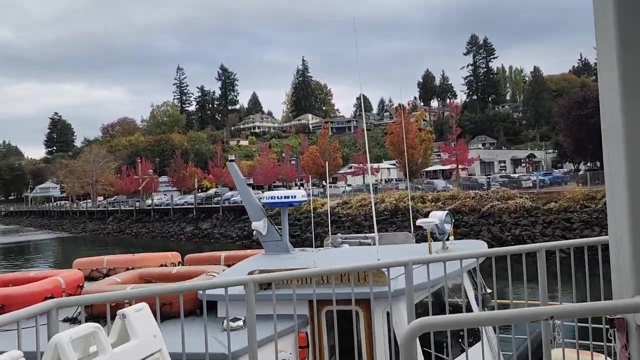 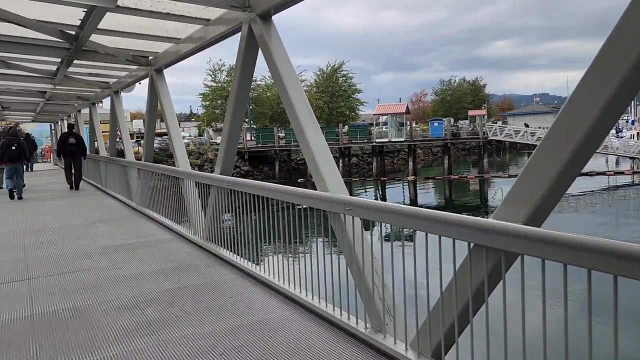 It opens to me. So I'm finally in Port Orchard. where's Joel? Huh, Look at this. it's so beautiful. Wow, They're really starting to turn now. Yeah, Back in Port Orchard.